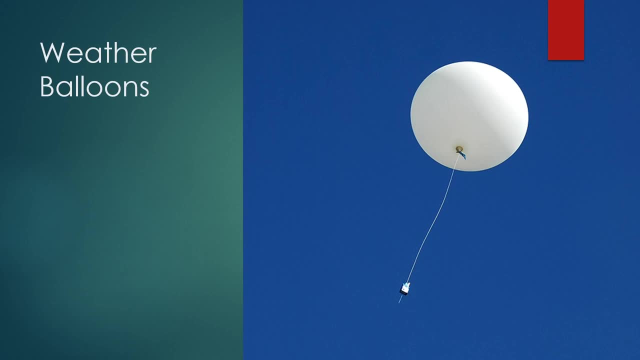 Before getting into that, let's talk about weather balloons. Two times a day, at around 0 UTC and 12 UTC, which UTC is commonly referred to as Z or Zulu in the meteorological community, weather balloons all around the world are launched. 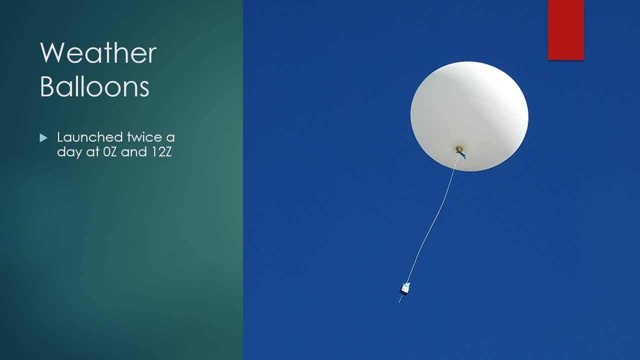 In total, there are over 900 balloons that are launched twice a day, including 92 that are launched by the National Weather Service. The weather balloons have instrument packets attached to them, which have a thermistor to measure the temperature, a hygristor to measure the humidity and an aneroid barometer. 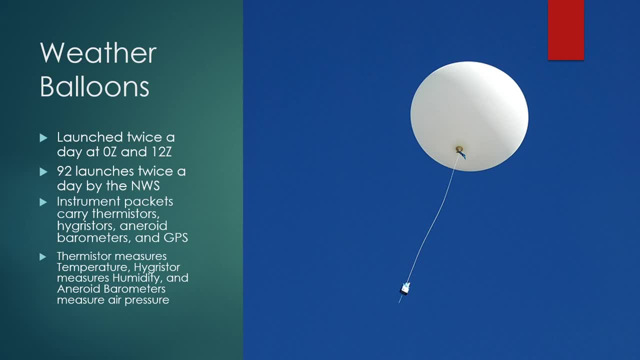 to measure the pressure. They also contain a GPS and the GPS is used to measure the wind speed and direction and the height of the balloon. As the balloon moves up through the atmosphere, it gets moved by the wind and the GPS tracks the path of the balloon. 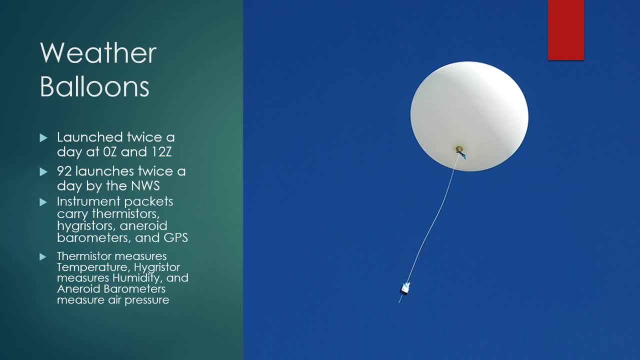 versus the time, which will tell you the wind speed and direction at certain heights. These packets of instruments are called radiosondes. These radiosondes send the data back to the National Weather Service, which is then packaged and released to the public on the SPC's website. 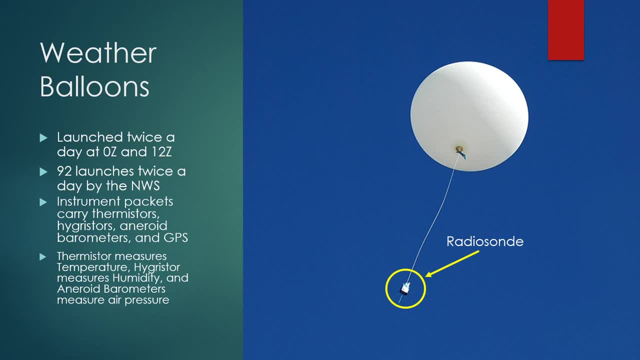 and is sent to the National Centers for Environmental Prediction, or INSEP for short, where the data is then used to initialize weather models like the NAMM model or the HRRR model. The data that is gathered from the radiosondes are usually plotted on Skew T log P graphs. 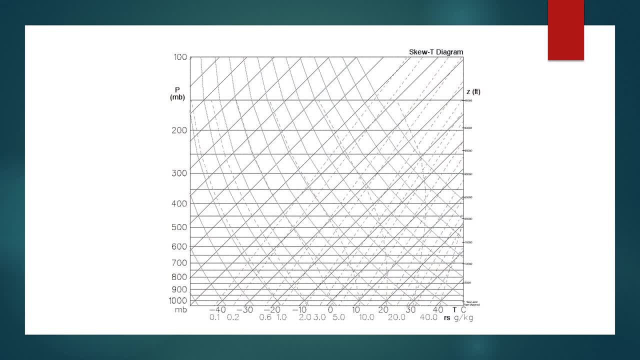 Skew T's are good for a variety of reasons. First of all, they have numerous lines on them that are great for thermodynamic analyses of the atmospheric profile. It is called a skew T graph because the temperatures on the graph are skewed to the right. These are the 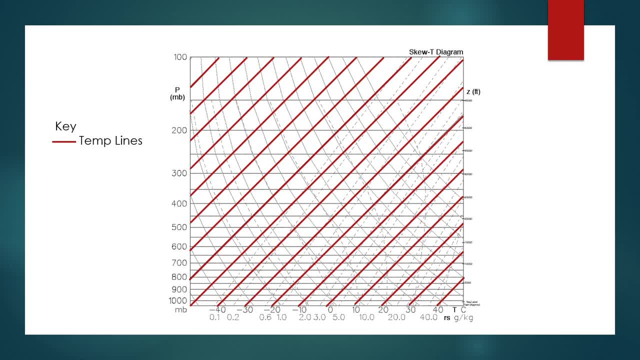 temperature lines. This is particularly helpful because almost the entire radiosonde sounding is able to be plotted on the graph. If the temperatures weren't skewed to the right, the temperatures might clip off the edges. The second part of the skew T graph is log. 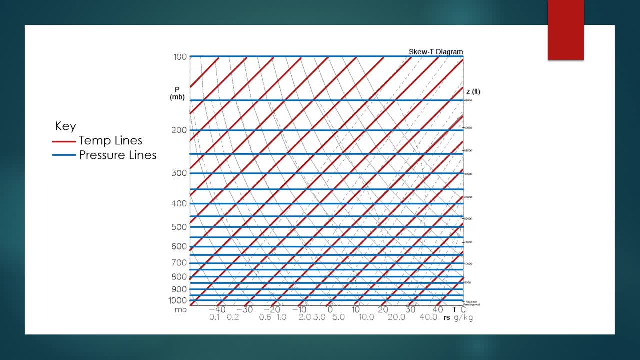 P. This is the temperature line. This is the temperature line. The temperature line is the temperature line. This is because the pressure decreases logarithmically with height. The atmosphere is compressible, and so there is a lot more air near the surface than there. 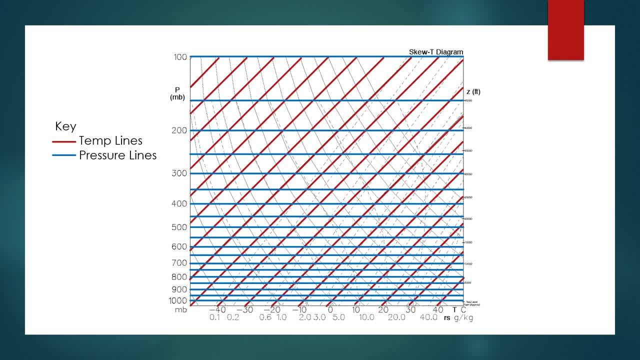 is very high up in the atmosphere. The skew T graph is representative of that. The compression of the atmospheric pressure near the surface on the skew T is important because features near the surface, where most of the weather happens, are exaggerated, which helps meteorologists and storm chasers notice features we would otherwise miss. 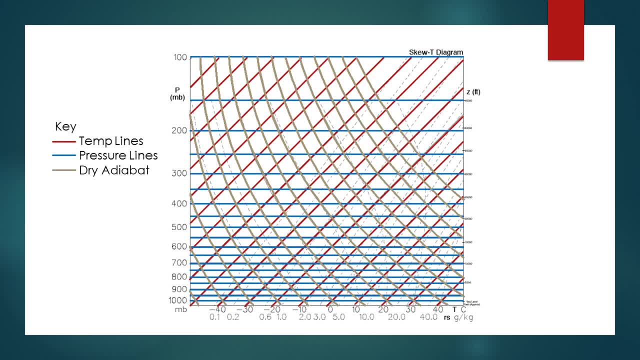 The third part of a skew T graph are the adiabats. First we'll look at the dry adiabats shown here. These curved lines are the paths that parcels of unsaturated or dry air would raise in the atmosphere due to lift or convection. 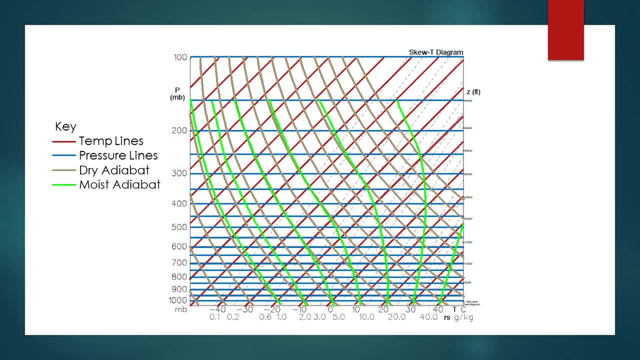 Next are the moist adiabats, which are sometimes referred to as saturated adiabats. These are the paths that parcels of saturated air would rise in the atmosphere due to lift or convection. I'll talk more about differentiating a dry or saturated parcel later. 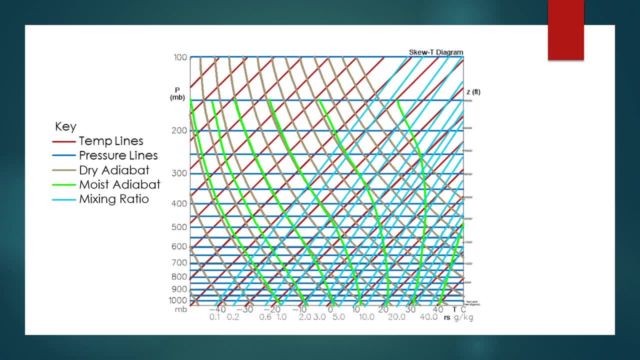 The last part of the skew T plots are the mixing ratio lines shown here. These are the mixing ratio lines. The mixing ratio lines are helpful for identifying the lifted condensation level, which is important for calculating convective available potential energy, or CAPE for short. I'll discuss CAPE in my next video on Friday. Mixing ratio. 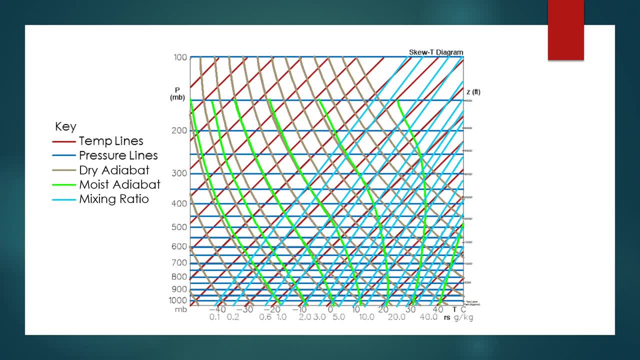 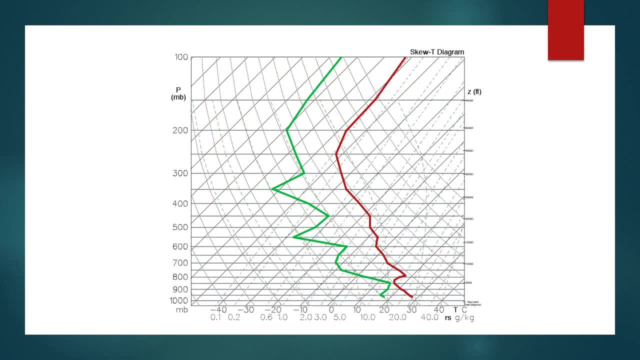 is also important when determining the wet bulb temperature. It's an important part of determining whether a parcel is saturated or not. This is an example of what a skew T might look like. The red on the right is the environmental temperature profile. This is the temperature that the radiosonde measured during its 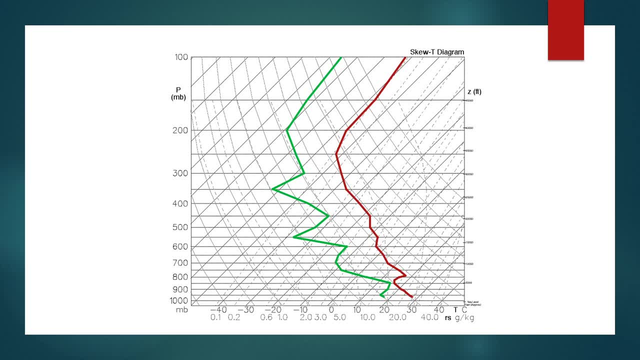 descent. The green line on the left is the dew point profile that the radiosonde measured. If, at any point, the dew points and the temperatures meet, this is where the air is saturated and you will likely have clouds. Another product you can determine, as I mentioned earlier, is the lifted condensation level. 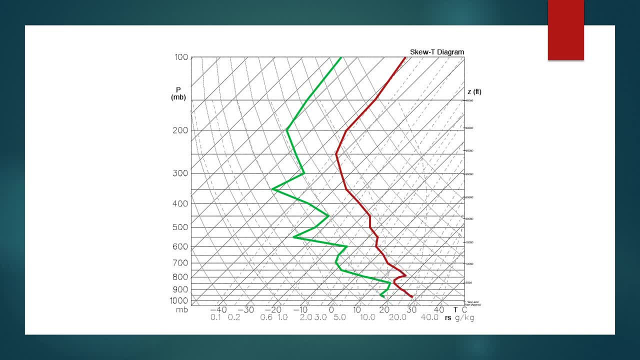 or LCL for short. In order to determine this, you take the surface parcel located here. This surface parcel is a dry parcel, it's not saturated, so you follow it up the dry adiabat line And if there isn't a dry adiabat line right on the surface parcel, you can make your. 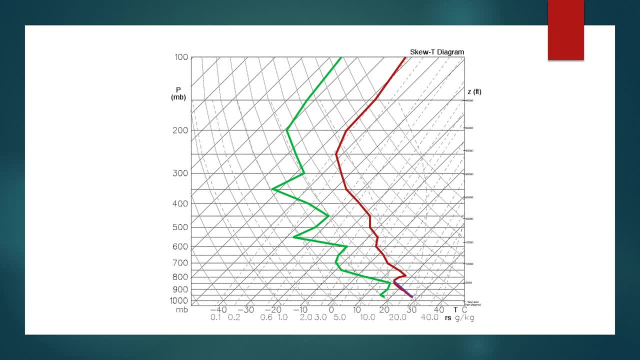 own, following the path of the other dry adiabats. Then you take the surface dew point temperature and follow it up: a mixing ratio line. Now, if there isn't a mixing ratio line, once again, you can make your own, following the path of the other mixing ratio line starting from your surface dew point.